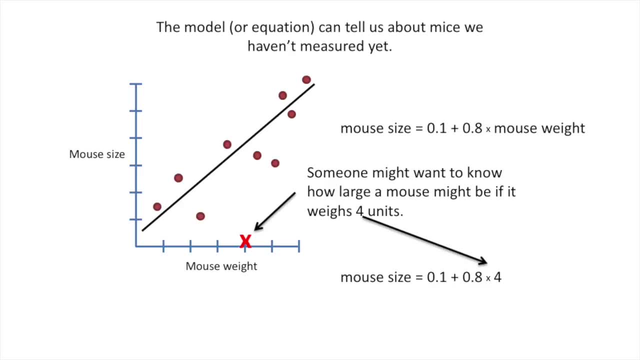 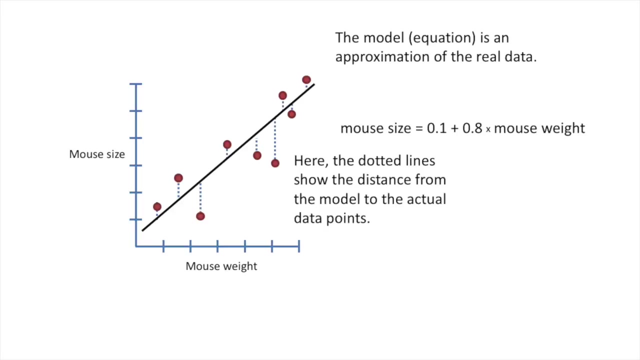 if it weighs four units. So we plug that value into our equation and we get mouse size equals 3.3.. The model predicts that a mouse that weighs four units will be 3.3 units big. The model or equation is an approximation of the real data. Here the dotted lines show: 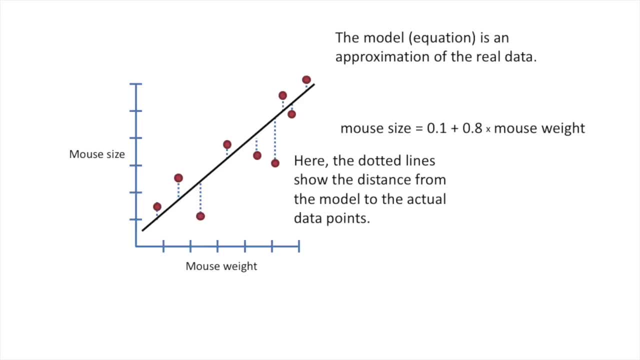 the distance from the model to the actual data points. A lot of statistics is dedicated to determining if a model makes a good or bad approximation of the data. Right now I'm working on a bunch of new stat quests to cover these subjects specifically. This includes 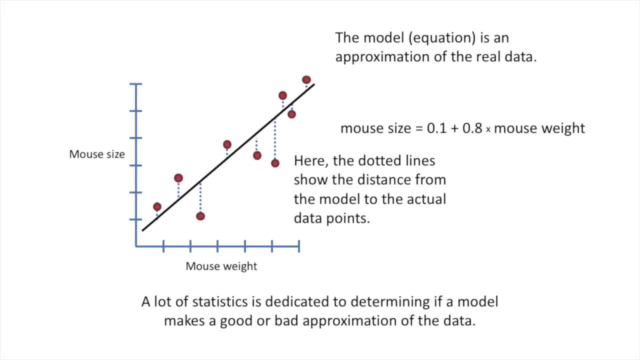 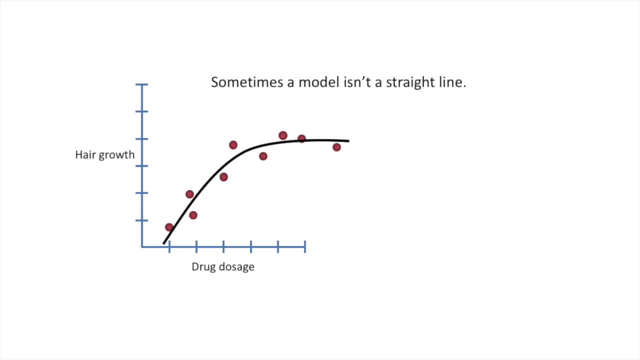 linear regression, general linear models, t-tests, ANOVAs and F-tests and all kinds of really exciting things that I can't wait to cover. Sometimes a model isn't a straight line. In this case, the model helps us understand the relationship. 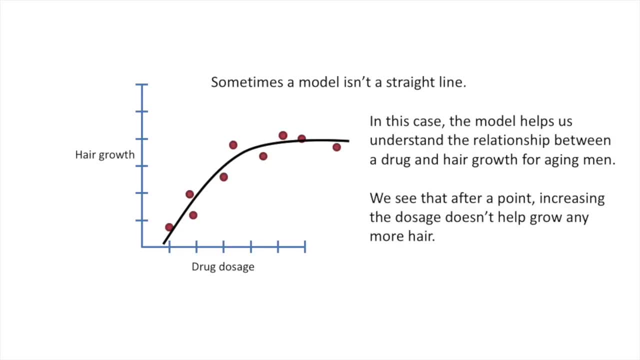 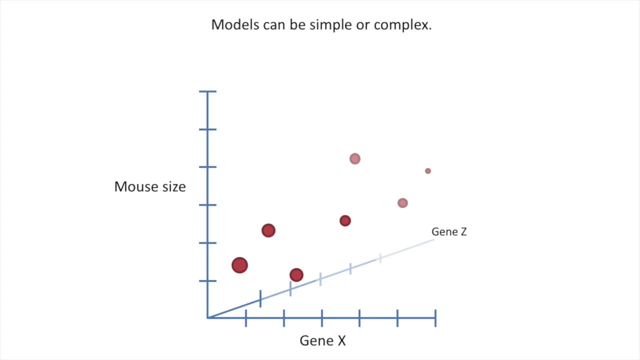 between a drug and hair growth for aging men. We see that after a point, increasing the dosage doesn't help grow any more. hair Models can be simple or complex. Here we are using two genes, X and Z, to model mouse size. 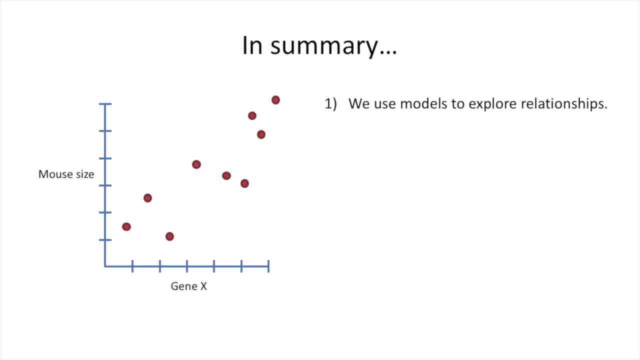 In summary, we use models to explore relationships. For example, I might be interested in the relationship between gene X and mouse size. We then use statistics to determine how useful and how reliable our model is. Hooray, We've made it to the end of another exciting stat quest, If you like this stat. 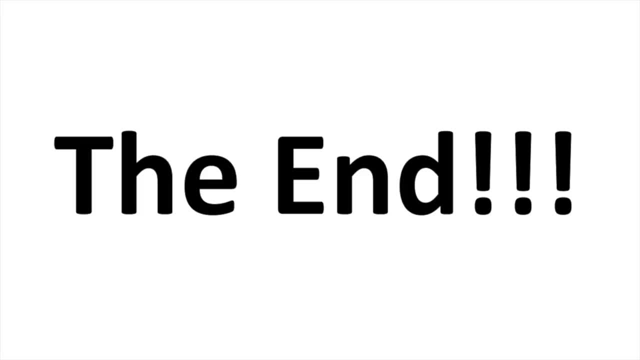 quest and want to see more of them, please subscribe, And if you have any stat quest ideas of your own that you'd like me to cover, just write them down in the comments below. Alright, tune in next time for another really exciting stat quest.